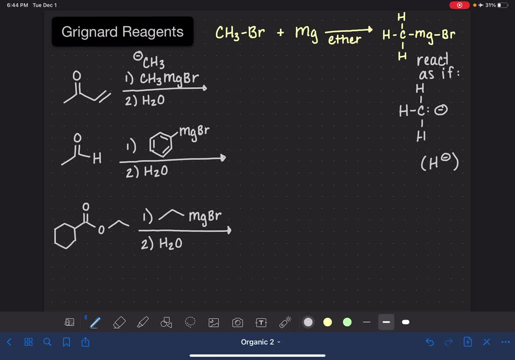 reagent as just an alkyl group with a negative charge on it, Like a hydride reagent. that negatively charged alkyl group is going to attack the carbon of the carbon oxygen double bond and it's going to cause that bond to open up. This is going to create just like with the 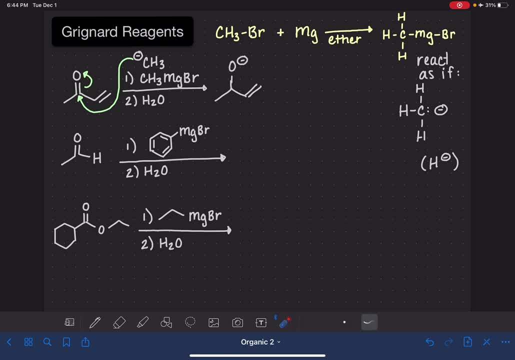 hydride reagents. it's going to create an OH- And this R group from the Grignard, in this case a CH3 group, is going to attach itself to the carbon of the carbon oxygen double bond. So we're creating a carbon-carbon bond. It might be. 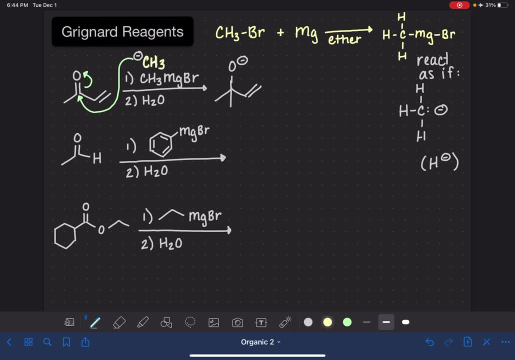 helpful if I do some color coding here, make this yellow, Just like with the lithium aluminum hydride reaction. step two of this reaction involves adding water to that intermediate, and the water is being used to put a hydrogen on the OH- This gives us an alcohol, This Grignard reaction, not. 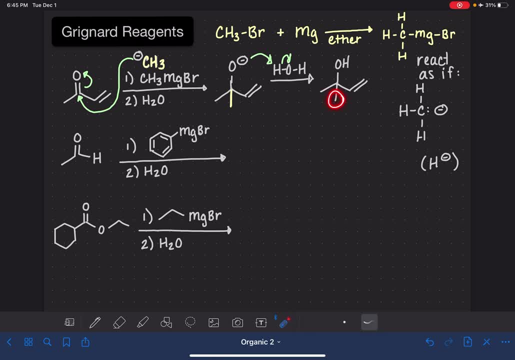 only does it add carbons to the original molecule, but it also converts the carbon oxygen double bond into an alcohol as well. Here's another example: In this situation, we're looking at reacting our Grignard with an aldehyde instead of a ketone and we have a much different Grignard reagent. 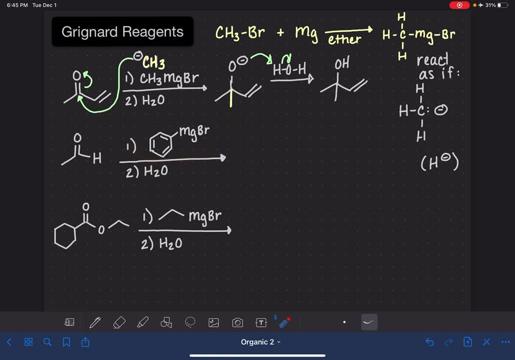 There's a lot of variety, So for this particular one, we want to be thinking about it like this benzene ring that has a negative charge on one of the carbons in the benzene ring. That negative charge is going to attack the carbon. 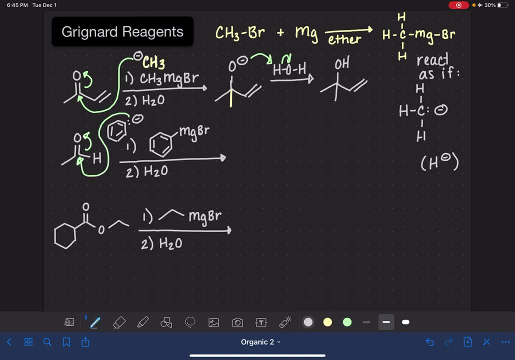 of the carbon oxygen double bond open up that double bond. So we're going to get an intermediate that will be a carbon-oxygen double bond, and then we're going to have a carbon-oxygen double bond that will be a carbon-oxygen double bond. So we're going to get an intermediate that. 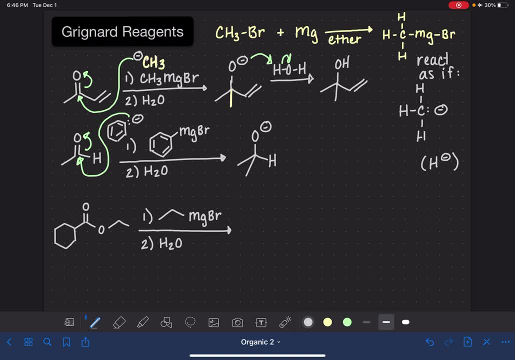 looks like this and we will have formed a bond to that carbon atom. the carbon oxygen double bond. carbon atom from that benzene ring added that whole entire thing to the molecule. then again, in step two, we're just going to be using water to protonate our O- to create an alcohol like that. our last example: we have a. 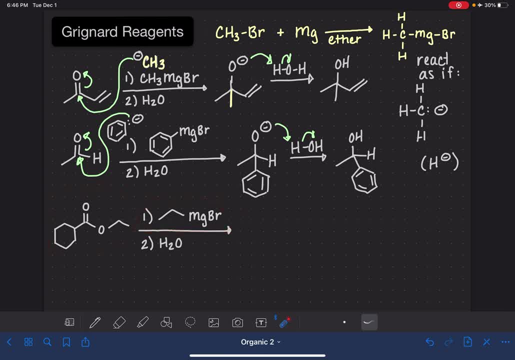 smaller Grignard, this time reacting with an ester. and in this reaction again we want to think about our Grignard as a carbanion, a negative charge on that carbon. it is going to be attacking the carbon-oxygen double bond, opening up that bond. now. we have in the past looked at hydride reagents reacting. 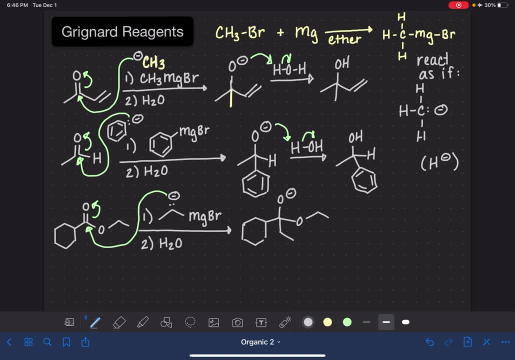 with esters. this is going to be a really similar process when you're adding the Grignard. so we're adding a two carbon Grignard, make sure you get both of those carbon atoms added to the molecule. this in this particular mechanism, because we're starting with an ester, things look a little bit different. aldehydes and. 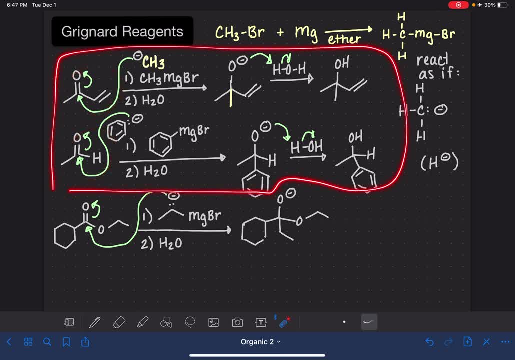 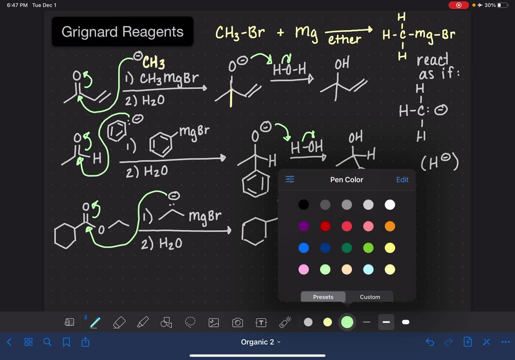 ketones always react in this particular way. just to give you a little bit of an idea of what we're going to be doing next: just like a hydride reagent, but esters react a little bit different, like we've already seen with hydride reagents. so in our next step we're going to bring 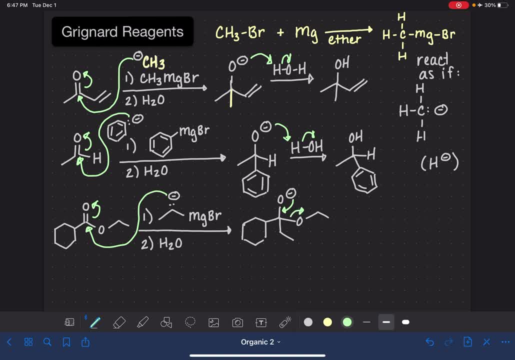 those electrons back down and reform the carbon-oxygen double bond and we are going to get rid of the O-R group from the ester. it gives us this guy. now I've kind of rearranged the positioning of these two carbon atoms in the molecule. I've moved them and I'm going to put them back together and then I'm going to 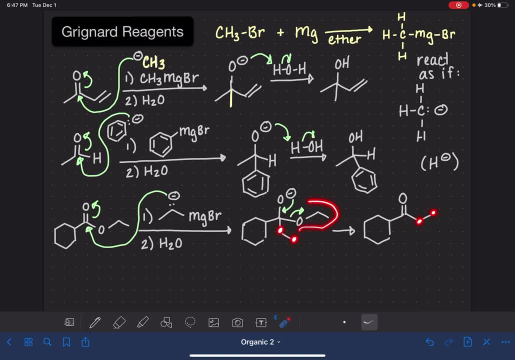 move them just to kind of make it look symmetrical and pretty. so I got rid of this. we've got this O-E-T group that's gone from the molecule and we're not going to draw it anymore because it's not, it's not an important part of the 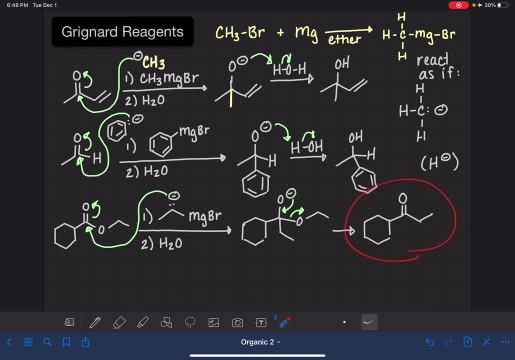 molecule. when we get to this point, this reaction is- you know it's- very favorable. so we're actually going to get a second Grignard in the mix. I'm gonna bring in Grignard number two. still want to think about it like a negative charge on the carbon. that Grignard is going to attack the carbon of the 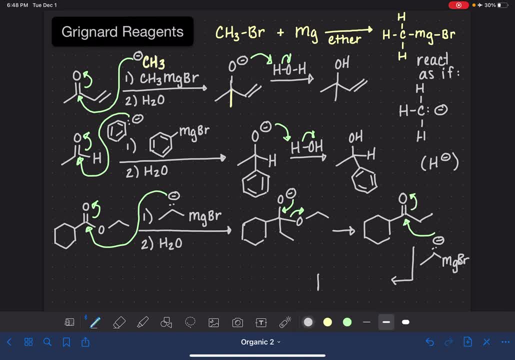 carbon-oxygen double bond, so we're just kind of repeating this process. a second time we saw the same thing happen when we were doing hydride reagents on an ester, so we've added two at this point. we've added two of the R groups from the. 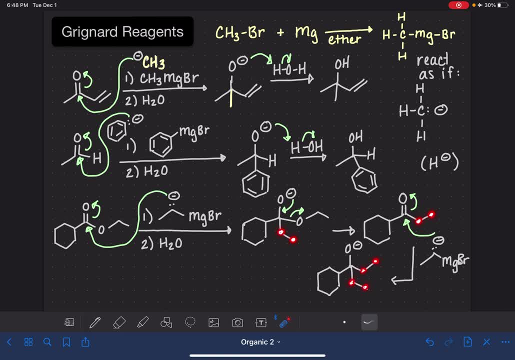 Grignard, I've got one there and then here we've brought in our second to R group. now, when we get to this point, when we've added both of those- our groups- the the last thing that happens, just like with the lithium aluminum hydride reaction.